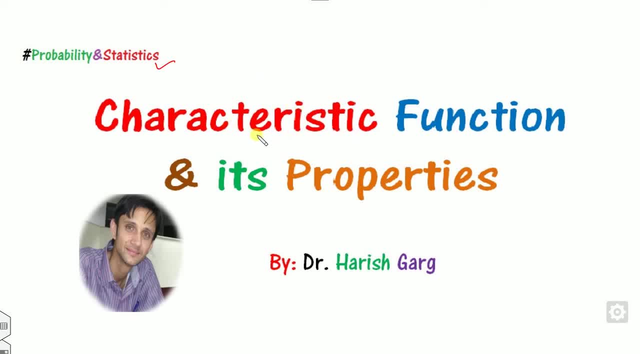 Hello everyone, welcome to the next lecture on the probability and statistics. In this class we will see what is the characteristics function and what are the various properties. Myself, Dr Gark, working in the School of Mathematics Thapar Institute, India. You can contact me as: 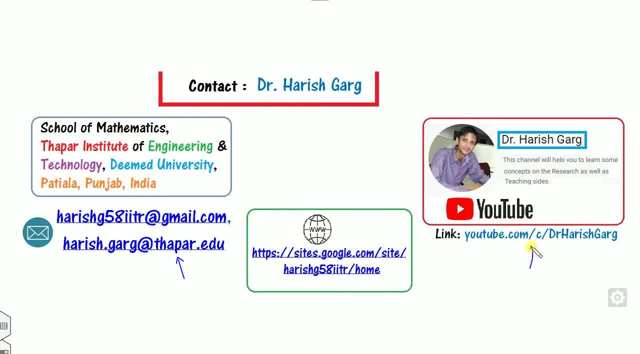 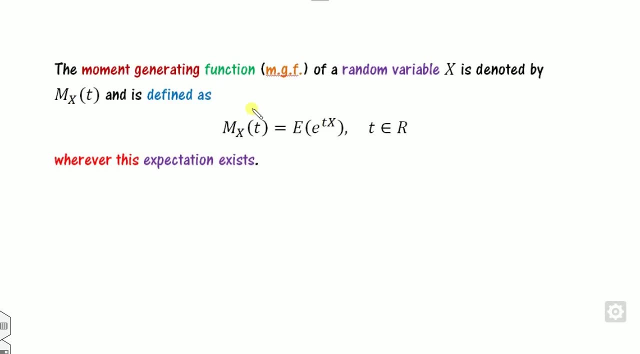 user through my either of the email ids or simply you can follow this link and the playlist related to the probability and statistics, where you can find the full course of this subject. Now, what we have studied so far related to these probability and statistics, and the moments are there. So 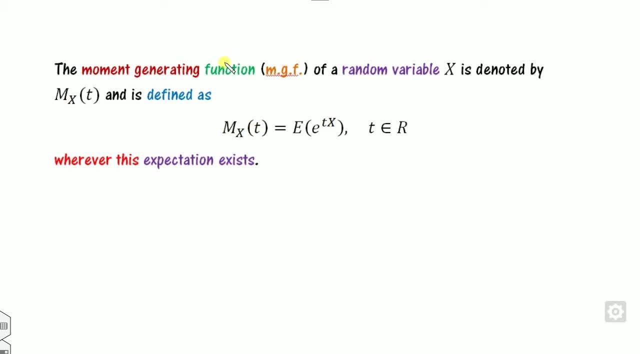 in the last lecture we have seen about the moment generating functions and clearly it is a function. So you can see that domain is from the real line to, since it is expected value, So it is again a real line. But another scene we have seen in the moment generating function lectures are that 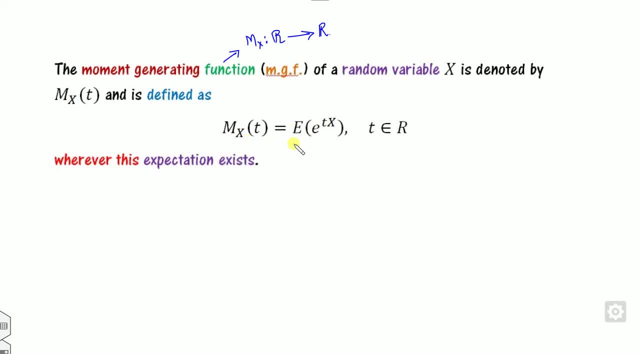 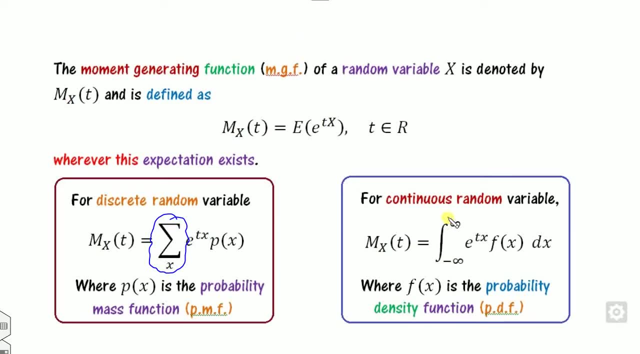 it has several shortcomings are there because this expectation- this is expectation- is depending upon the probability and statistics. So in the last lecture we have seen about the moment generating function, whether it is a discrete or continuous. So this summation, as well as this, 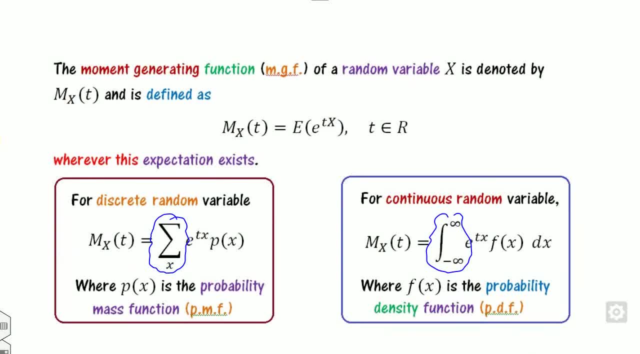 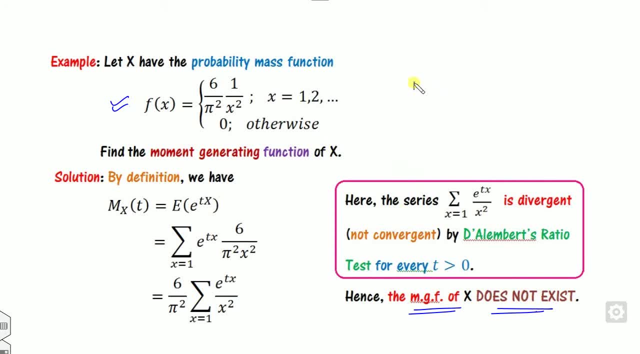 integration. it may or may not be converges, For example, if we have seen in the last class. if we consider this example, then the moment generating function does not exist. or you can say the moment generating function does not exist for all the values of the t, because my moment. 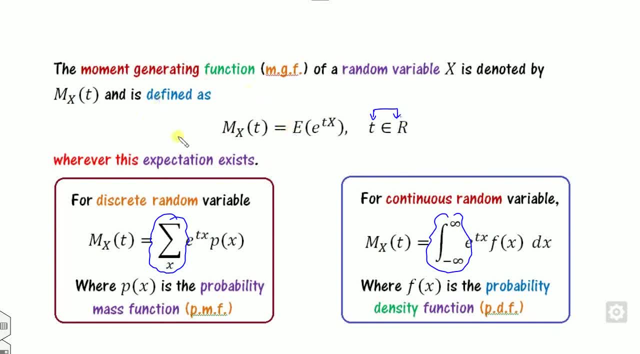 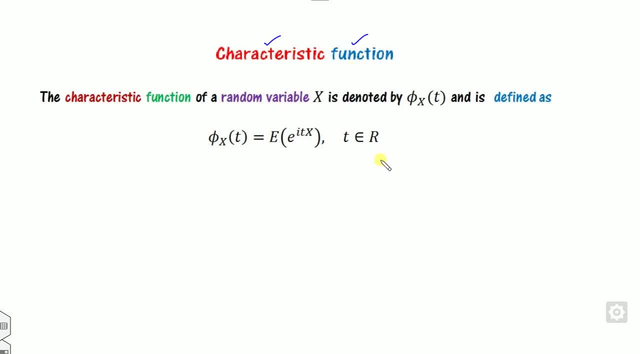 generating function is depending upon the this t. In order to overcome this drawback, there is another function called the moment generating function. So, in order to overcome this drawback, there is another function called as the characteristics function that came into the feature and that's the topic of our today's lecture. So what is the moment? what is the? 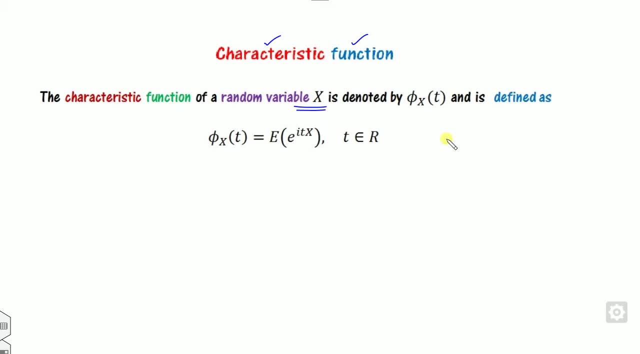 characteristics function. is that characteristics function of the any random variable x. it is denoted as a phi of x. Again, it is a function. So you can clearly see that. what is the domain of this? it is defined on the small t. So it is from the real line to now, since it is expected. 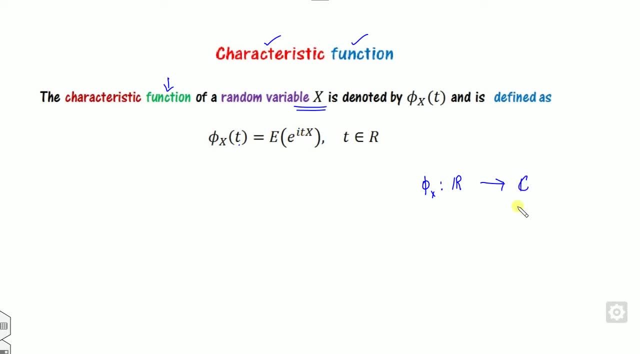 value of year iota. So it's a complex plane. So you can say this: it is a complex plane, So you can say: this is the r to the c. So once you are knowing the value of the expectation, then you 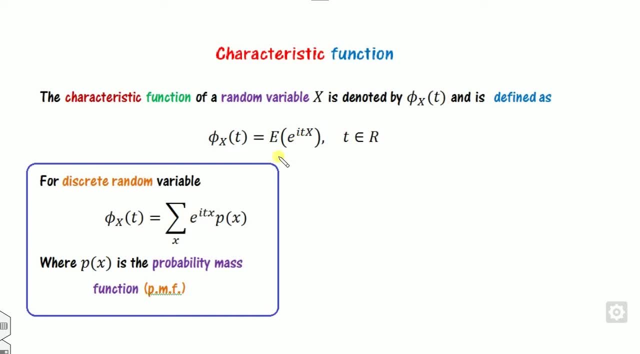 can, as usual, define the discrete for the summation sign for e raised power. iota tx of p. p is nothing but probability mass function. On the other hand, if it is continuous, then you can define like this way: Now the major question arises: is that what is the necessary and the sufficient condition for? 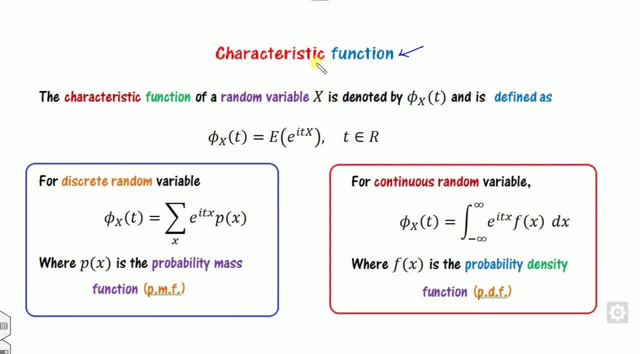 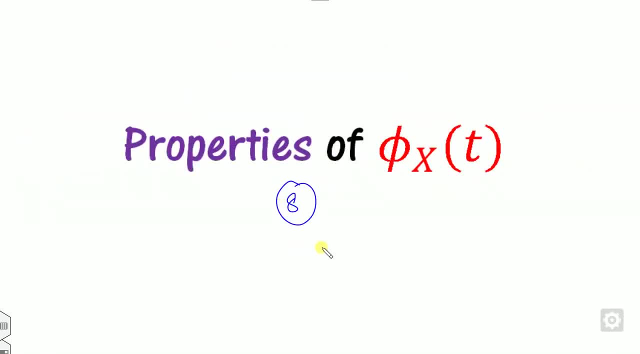 this characteristics function, Before defining the necessary and sufficient condition, we must satisfy certain properties For this characteristic function that we will discuss here. So we will discuss eight properties for this characteristic function, as here The first, most important property is that this characteristic 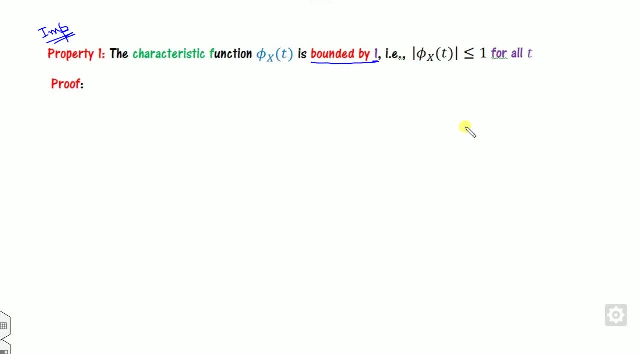 function is bounded by one. What is the meaning of the bounded is if, if I say this function is bounded, it means the modulus of this must be less than of one. The proof is quite trivial. You can see. start from this. since it is a bounded by one, So let assume x is a continuous. Later on we will. 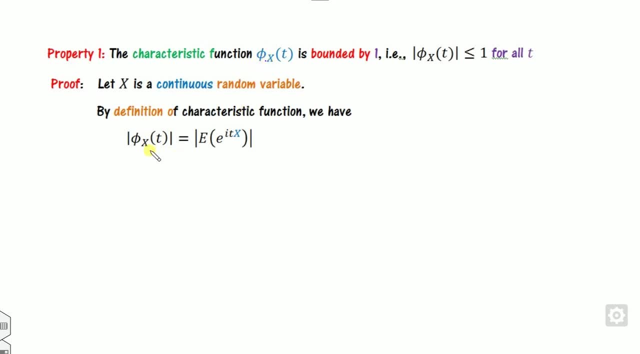 discuss for the discrete also. So by the definition of the characteristic function we can start with here. Now, what is the definition of? if it is a continuous? we can define this expected value like this way, And all of you know that: what is the integration of modulus, of the integration, it will. 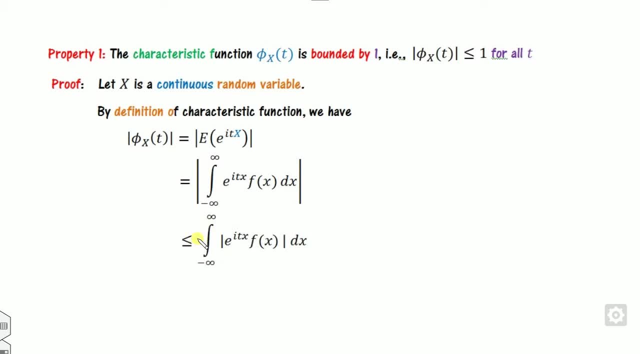 be less than of the integration of their modulus sign. So this is there. Now what is the integration of mod of a- b? Look at that. This is the first function, This is the second. It is nothing but my a and b Mod of a is mod of b. 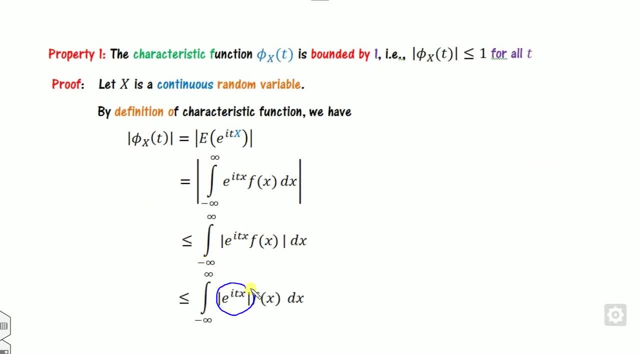 So you can define like this way: What is the modulus value of this here? So what is the modulus value of the z? It is always be a one, So you can write this as a one. Therefore, this Now: what is the p fx? This is nothing but the pdf And integration from minus infinity to plus. 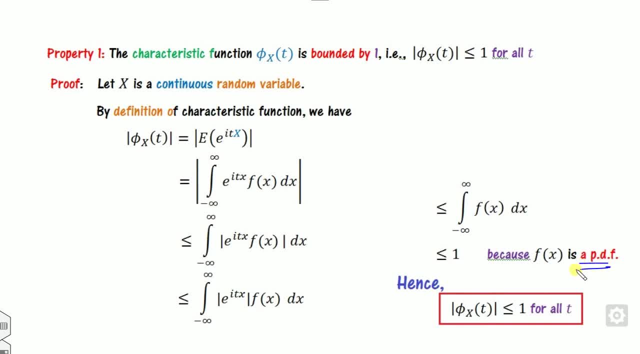 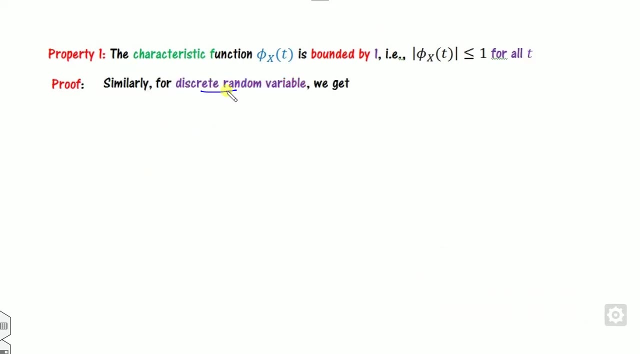 infinity pdf is nothing but one, because it is a pdf. Hence this mod of phi x is less than equal to one for all the values of the t. So therefore you can say: the characteristic function is bounded for all t. This is for the continuous. On the other hand, 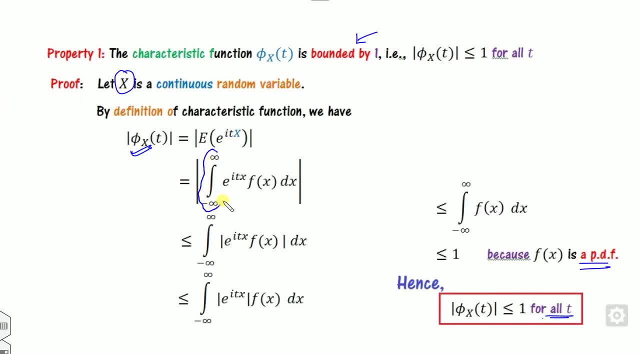 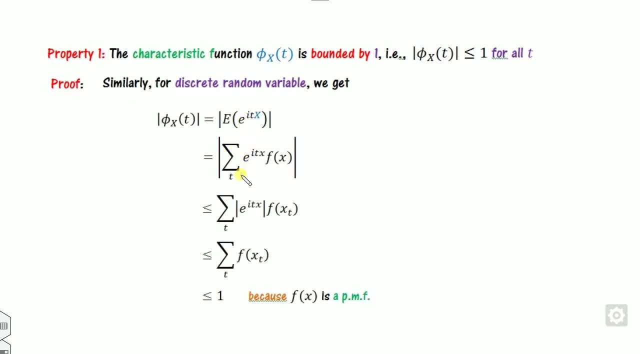 if it is for the discrete. what you can do is you can simply replace this integration to be a summation, this integration again to be a summation, and so on. You can see, the proof is quite similar. So here it is a pmf, So it is a. this summation is one, Hence this is bounded. Second remark is: 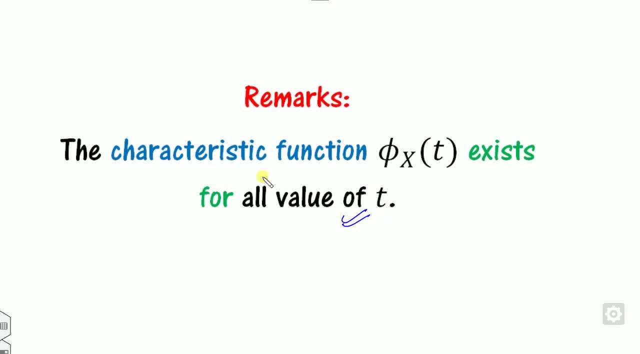 that you can see. the characteristic function exists for all the values of the t because it is a bounded continuous. is there So? second property is that the characteristic function satisfy. this property is there. So this is one of the most important property that we will see what is the necessary. 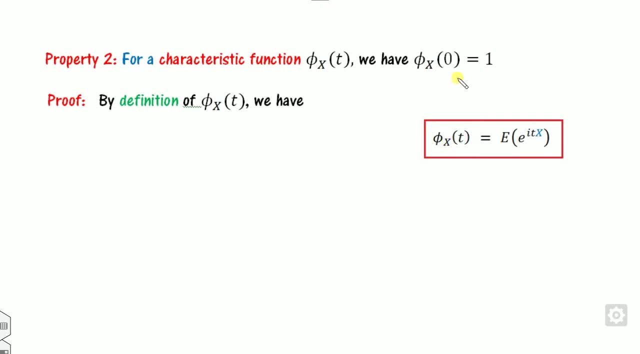 sufficient condition here. So again, it is clearly sees from the definition. So look at that. you can substitute small t is zero here What you will get? E raised power, iota, t, f. What is the this value is? This is nothing but my one. So that is a quite simple proof of this property. Second, third proof: 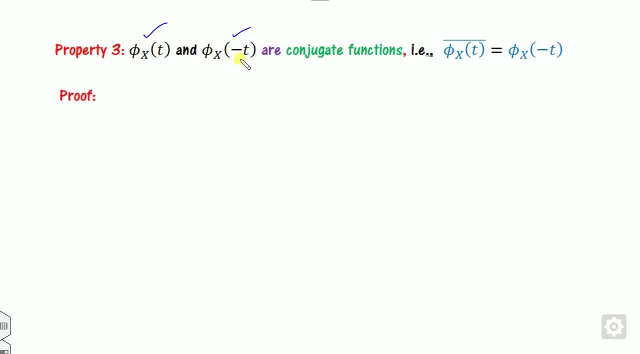 the most third important property is that the phi x and because it is a complex function. So phi x and phi of t are conjugate functions. The conjugate function means they are here. So once how you can prove that. you can start from this left hand side by the definition of the characteristic function. 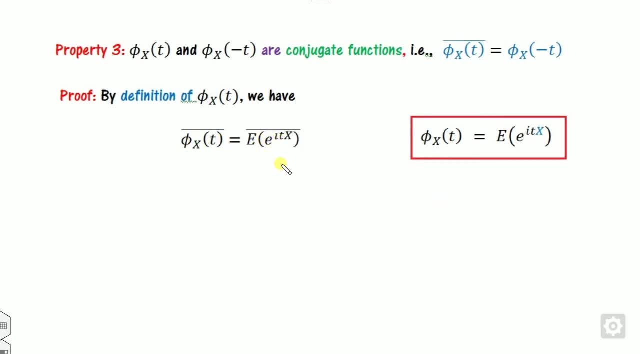 What is the modulus of this? So you can see this, how you can open this of e, of this. You can write like this way: What is the modulus value of this? If I say this is a plus iota b, then what is the? 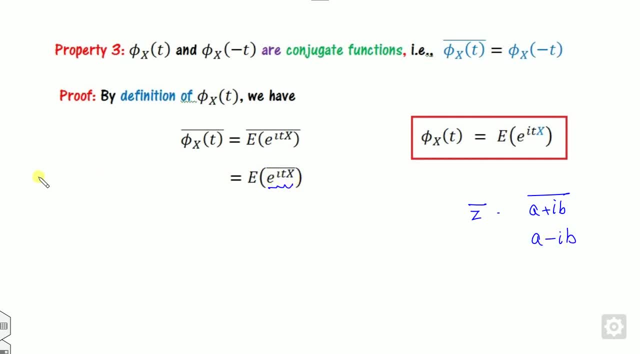 modulus of this is a minus iota b. So what is the modulus of this? So what is the modulus of this? What is the conjugate of this? So this is nothing but here. So if you compare this with the help, 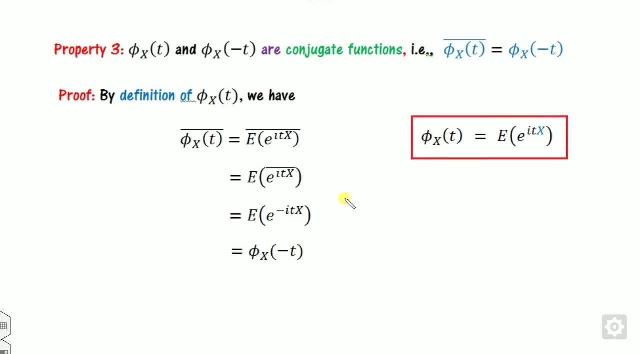 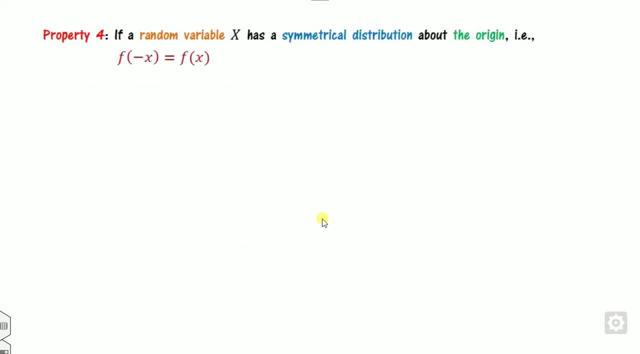 of this. what is that? This is nothing but my phi of minus t. So therefore this property also satisfy and we called, as they are, conjugate functions. Next important property is that if a random variable, x, is a symmetric distribution about the origin, What is the meaning of the? 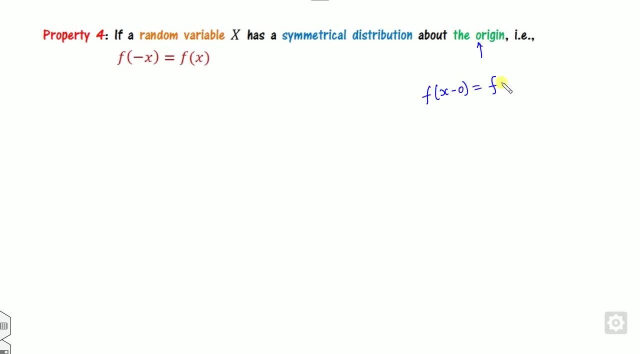 about the origin is If I say x minus zero, which is nothing but same as of minus of t, of x minus, because it is origin. So that is why zero. So you can write as f of x is equal to minus. 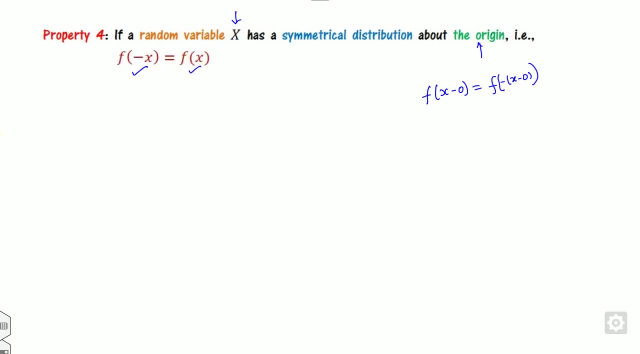 of x. So if any random variable x satisfy this property, then this phi of t, phi of x, that is a characteristic function, is a real value as well as the even function. So the proof is very easy, How you can prove that any function to be the even function. So if I prove that f of x 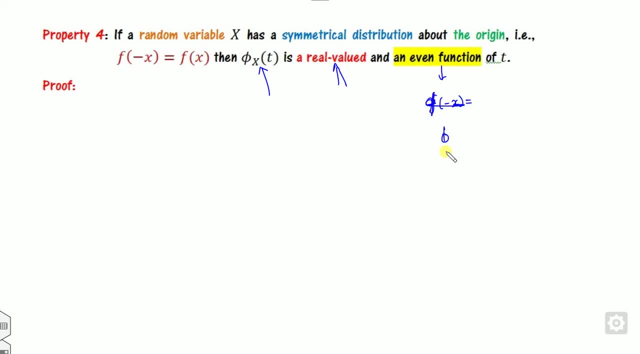 sorry, phi of x. So if I prove that phi of minus of t is nothing but my phi of t, then it is a even function And how you can prove that real value. So firstly we will prove that even function, So we can start for the continuous Discrete. 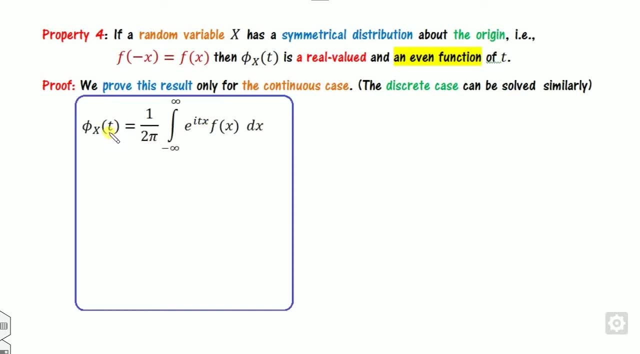 you can do easily yourself. So this is the definition of the characteristic function. Sorry, this is the characteristic function. phi of minus infinity to infinity. e raised power i over t x of f x. Now what is the value of the f? x Now if I, since f of x is minus f of? 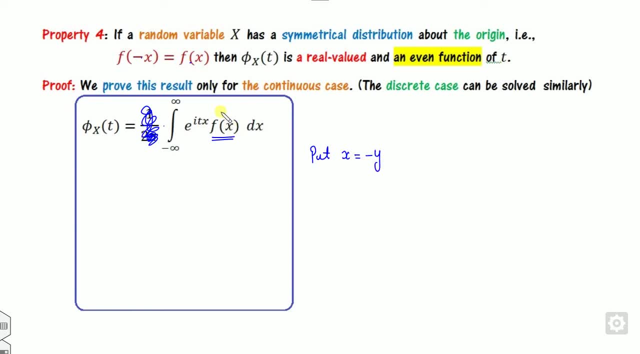 this. So if I substitute x is nothing but minus y, what will happen? What is the limit is So what is the dx is my, nothing but my, minus dy. So if you substitute here, limit will be plus. 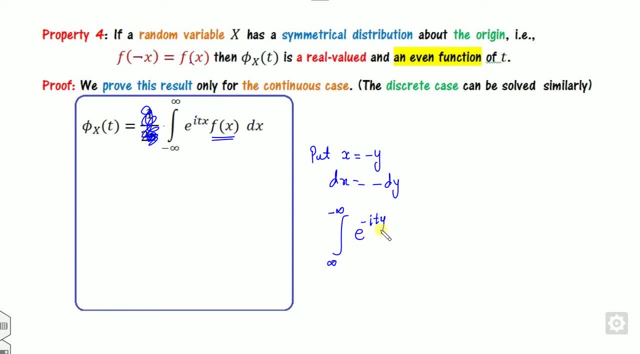 infinity to minus infinity. e raised power minus of this f of minus y, And this is minus of dy. Now for this minus I can adjust the limit. I can write here as this one. I can write like this way: Now f of x is nothing but minus y. So if I substitute x is nothing but minus y And this is. 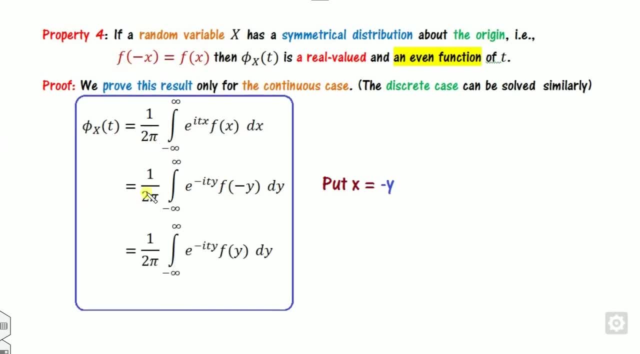 f of minus x is equal to f of x, So I can write like this way also. Sorry, this is not be there, So like f of minus x is nothing but here. So what is that? If you write this in terms of their: 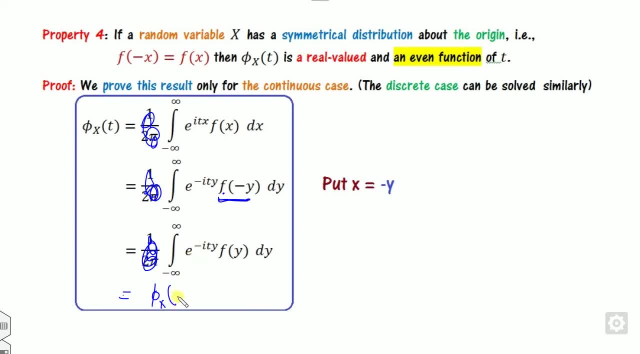 moment. in terms of the characteristic function, what is that? E raised power minus of t. You can see that. So, therefore, what is that is So? phi of t is nothing but phi of minus t. What do you conclude that This means? this is my even. 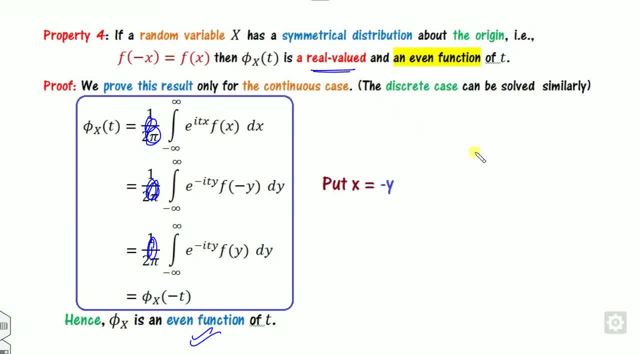 Second part, you have to prove that real value. So for any function, z, that is a complex function, when is said to be the real value. when z is nothing but my z, complex, It means the imaginary part will be zero. So if this condition holds, then your target will be the real value. So 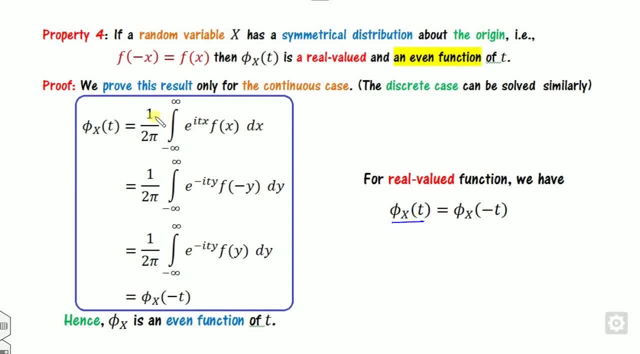 for this, what you can prove, that. You can start from here. Phi of x is nothing but here. because you have to prove that. And how you can write that. You can write this here, Why? Because phi x and phi of minus x are complex conjugates. So look at that. Phi and 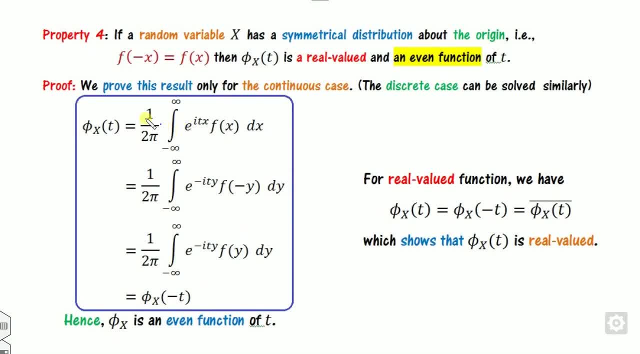 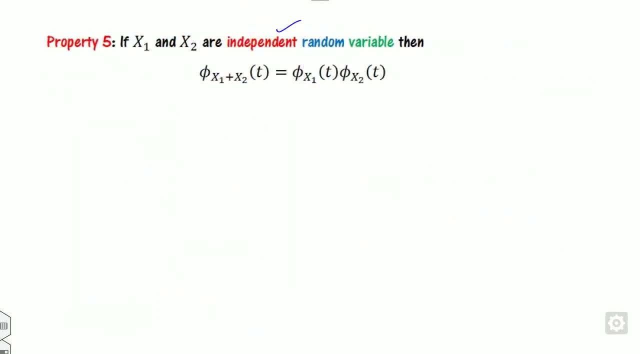 this are same. So therefore this is my real value function. Look at the next property. If x1 and x2 are independent, random variable, then this is there. So the proof is again trivial. You can start with the help of the phi. This is the definition. Now you can open this bracket. 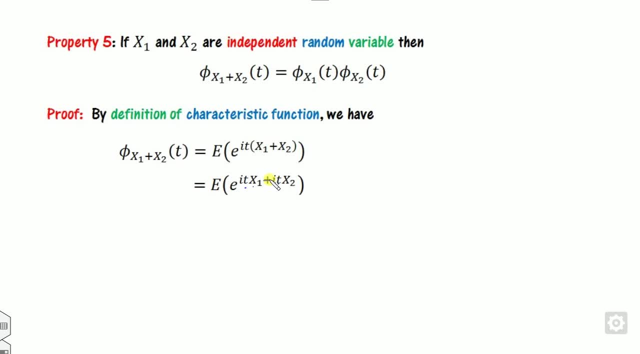 You can start like this way Now, since it is a multiply sign- sorry, it is a plus sign- So you can write in terms of this as product. So, since what is the meaning of the e, xy? if x and y are independent, random variable, then you can write as a product of: 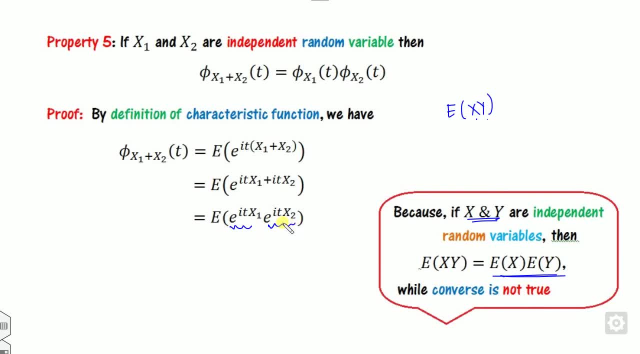 them, otherwise not So, since x1 and x2 are independent, so these are product. So you can write like this way. So what is the definition of this is: This is nothing but my phi of x1 and this is the phi of x2.. So therefore, the sum of the 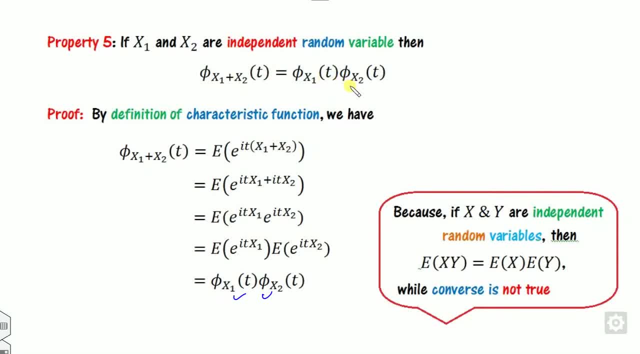 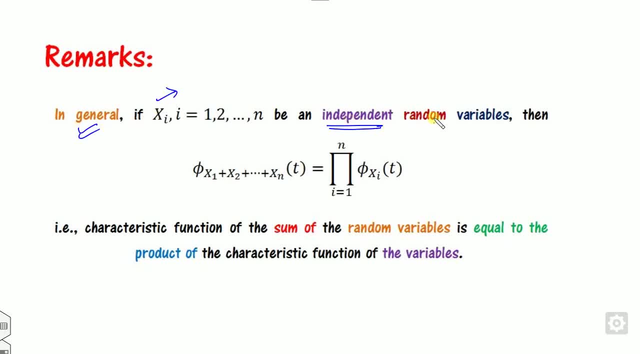 moment, generating function of this sum of the random variable is nothing but product of them. So this is for the two random variable. So remark is that if, in general, if xy's are my independent random variable, then the characteristic function of this sum is nothing but my product. 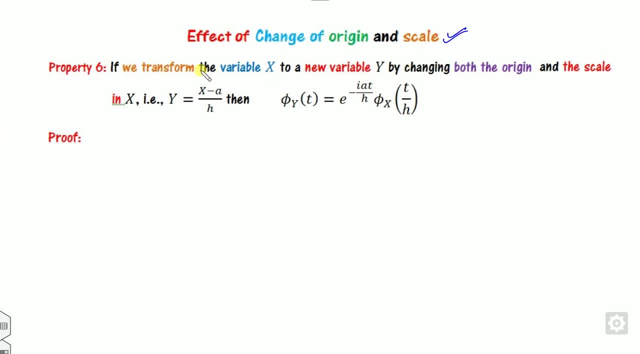 Next important property is the change of the scale and origins. So if we transform the variable x to be y, such that this y relation holds, then you can easily find the moment generating function of y like this. So we have already seen these properties for the MGF also, but now we can see how we can drive. 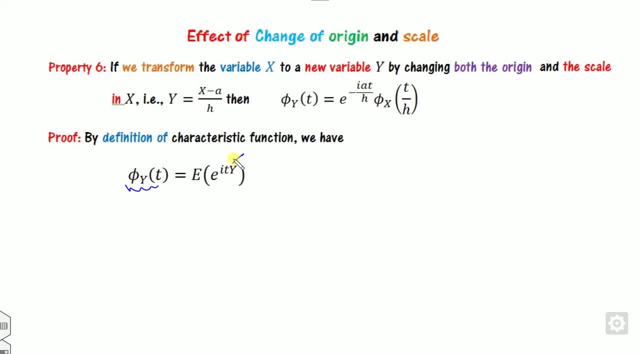 that. So you can start from the y. You can substitute the value of y here. This is the value of y You can substitute here. Now I can separate them. How you can separate them. This is there. So now, since this is the expected value, this is for the random variable x. So this part. 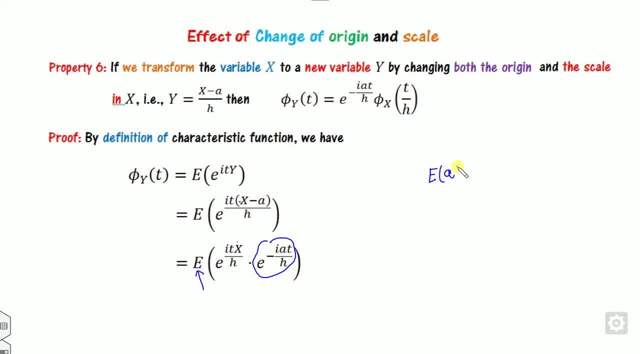 is a constant value, And what is the value of the e of ax If it is a constant? this is nothing but a of this. So this part can be taken as the outside. So this is there. So if you think about that, 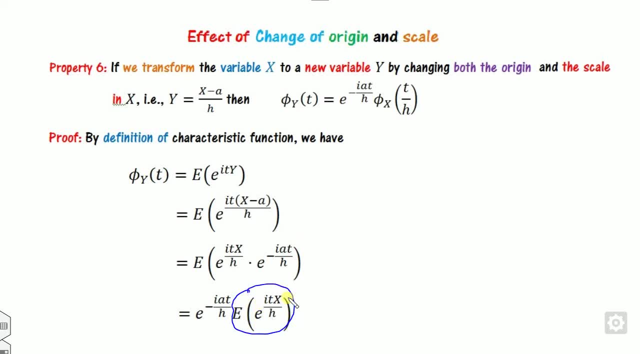 what is that? Is that definition of the characteristic function? Yes, So this is the definition of the characteristic function. with small t is my t by h, So you can see iota t by h. Sorry, this is not be the iota, This is t by h. You can see that is the quite. 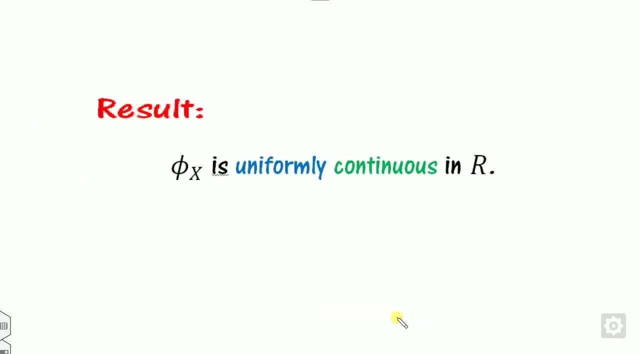 simple proof of them with the two, three lines, The seventh property, and you can this, you can prove yourself. So you can prove yourself. So you can prove yourself, So you can prove yourself. Well, for uniformly distributed, continuous function, but you can prove that you can start. 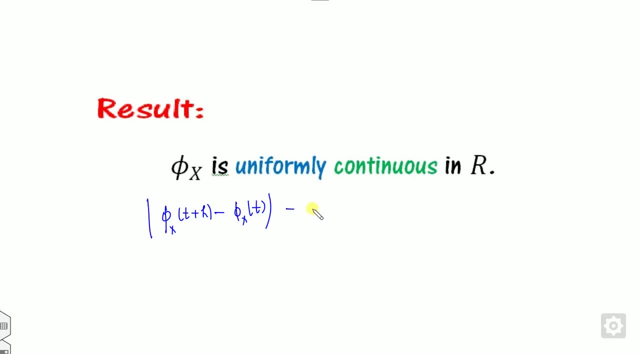 from here. Okay, You can start from here. If you can prove that this is approaches zero, as h approaches to be zero, then this function is my uniform, continuous, irrespective of their interval. h. Next property is that how you can find the mean of them if you have? 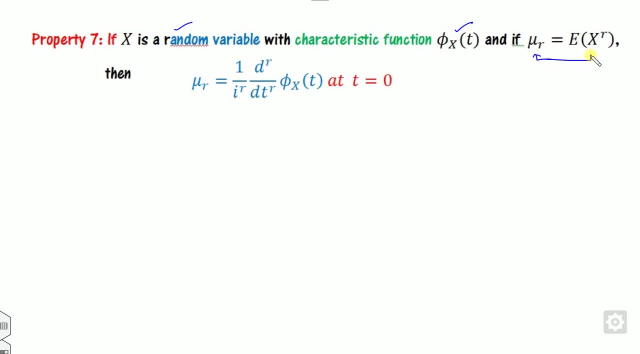 the x is a random variable for characteristic function y. These are general opinions from this future lecture, So we can start with some simple understanding of the definition of x. This is now, since we need the rth derivative, so you can derivative this r times with respect to the small t. So remember that with respect. 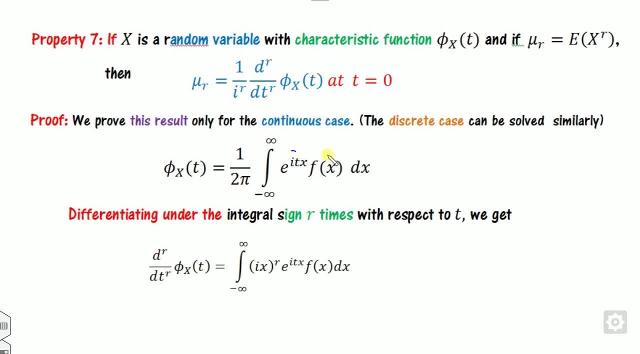 to a small t. this is nothing but here. So look at that. if you, since this part is constant, so what will happen? if you derivative this part as one time, so it will give you iotax. If you derivative again second time, so it will give you iotax. So what will happen? 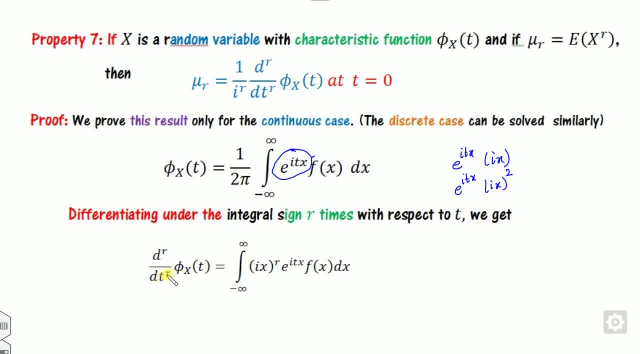 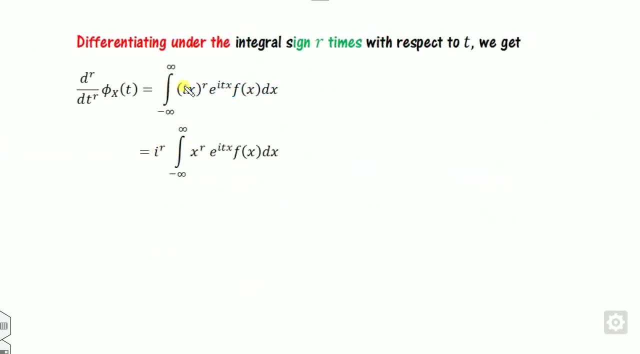 x, iota, x square and so on. so it means, if you derivative r times, it will give you here. now this integration is with respect to x. so you can write like this way: i raised power, r is taken outside iota, and what is that? nothing is there. so at t is equal to 0, what will happen on t: 0 left. 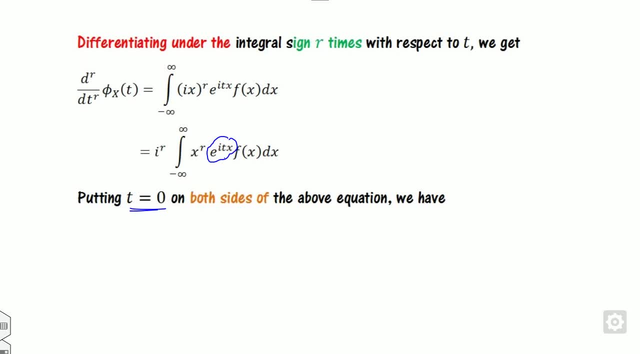 hand side. here this part will be my 1, so therefore this is here now. what is that can i write? is, as e raised power xr, because how you write the e of x square, this is nothing but minus infinity to plus infinity, x square, similarly so this is xr, so therefore i can write like this way here. so from: 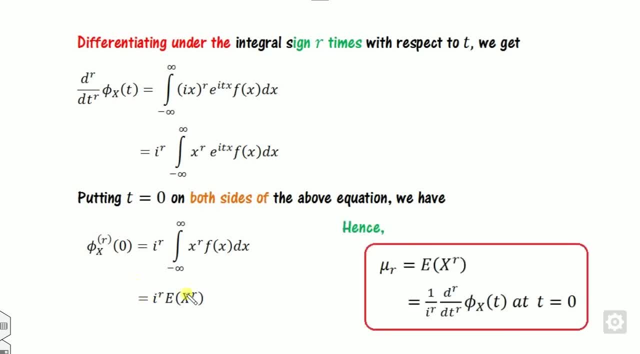 this you can find the value of this. this iota raised power r is nothing but the divided one. okay, so what is the meaning of this is: derivative value at t is equal to 0, so that's the derivation of this. the last property is the uniqueness theorem of the characteristics. 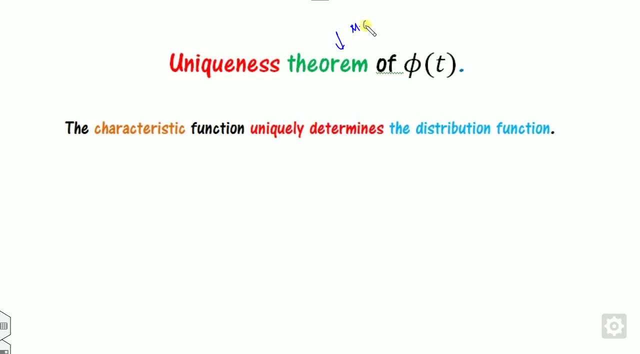 function. we have also seen the uniqueness theorem of the mgf, but right now we have seen the uniqueness property of the characteristics function. what it says? that the characteristics function uniquely determine the distribution function. what is the meaning is that if you have the two distribution functions or the two random variable x and y, such that the characteristics function of x and 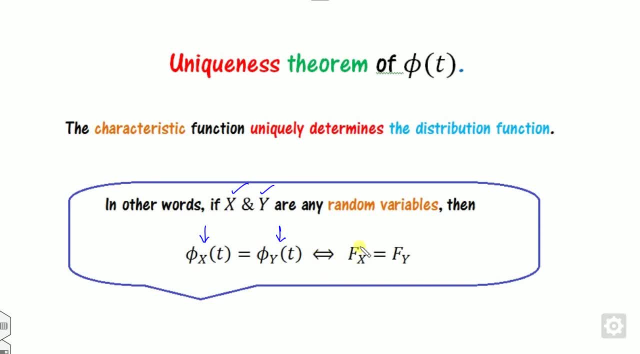 characteristics function of y are equal. it implies if, and only if, the cdf, that is the distribution function of x and y, is equal to 0. so that's the definition of the distribution function of x and y are same. or you can say the f of x is nothing, pdf of the x and pdf of y are same. or you can say 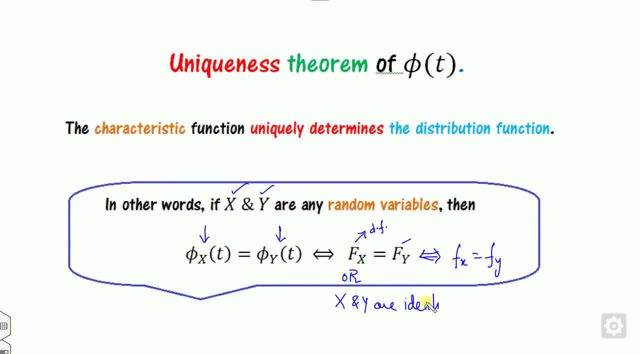 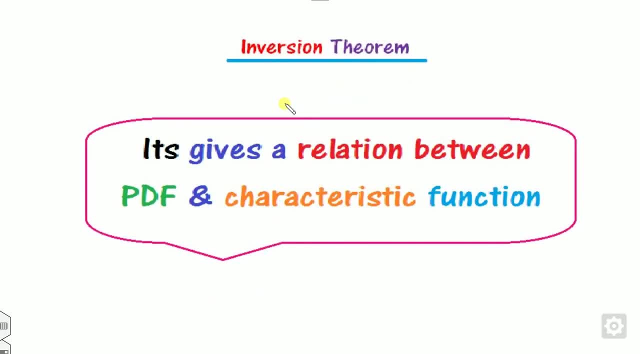 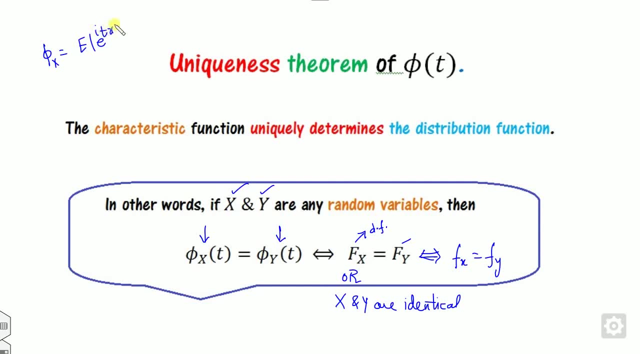 x and y are identical, So that we have also seen in the MGF property. The last one is the inversion theorem. What is that? You can see that what is the characteristic function is So if this here. So it gives you the relation between the pdf and it means if you have the 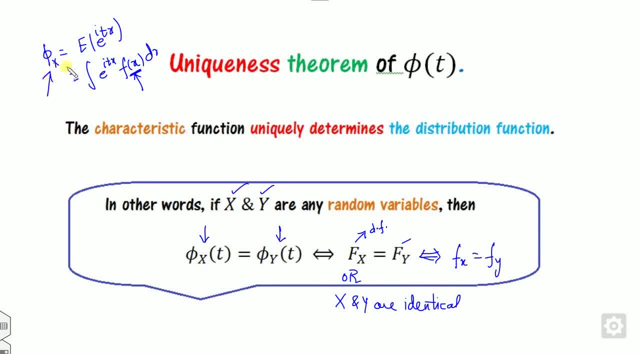 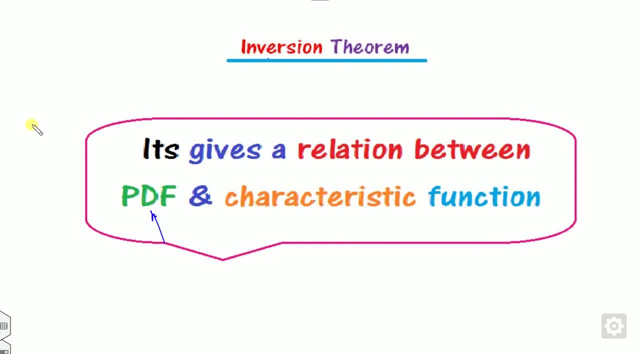 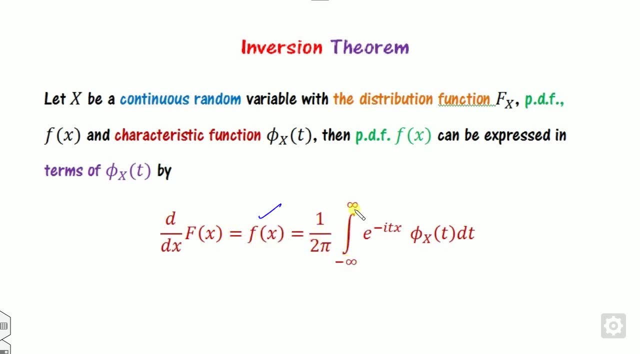 given probability density function, then you can easily find the characteristic function. So this inversion theorems give the reverse. You have to find the pdf with the help of the characteristic function. How Look at this? So f of x is nothing but 1 by 2 pi minus infinity to. 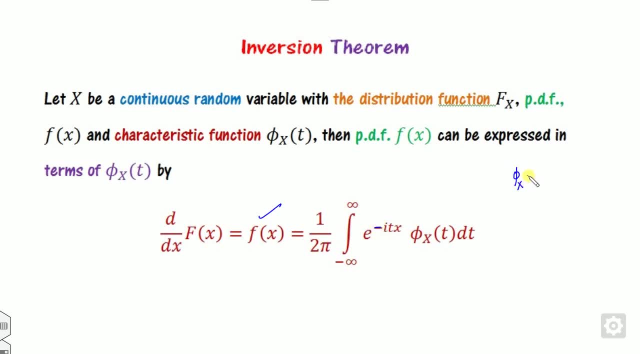 plus infinity. So if you have the probability density function, then you can easily find the pdf. Now look at that. This is the minus, because you can see what is the characteristic function is minus infinity to plus infinity of here. So remember this. it means f of x is given. 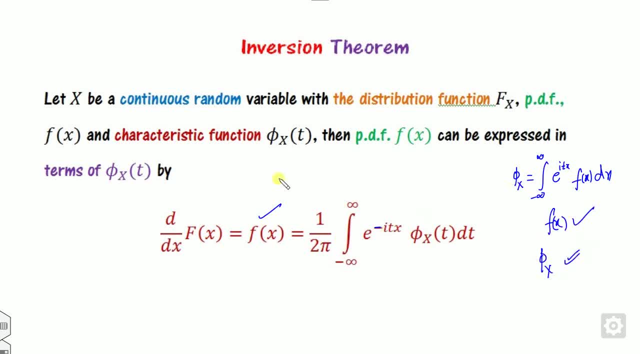 to you and you have to calculate the phi of x, But that's why this is called as the inversion. So this inversion means you have the given phi of x. Now, based on this phi of x, you have to calculate their pdf. So what is the meaning is: If x is a continuous random variable,